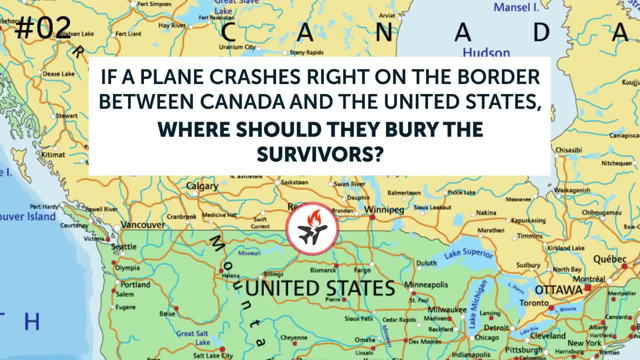 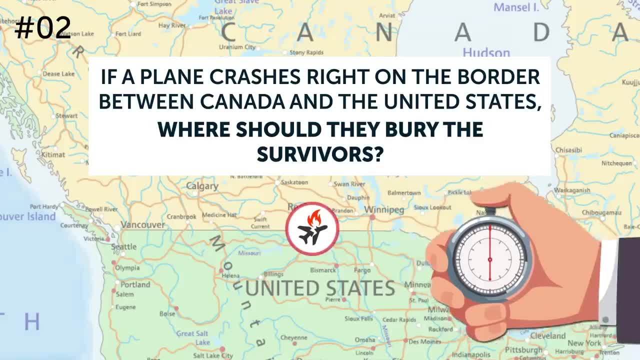 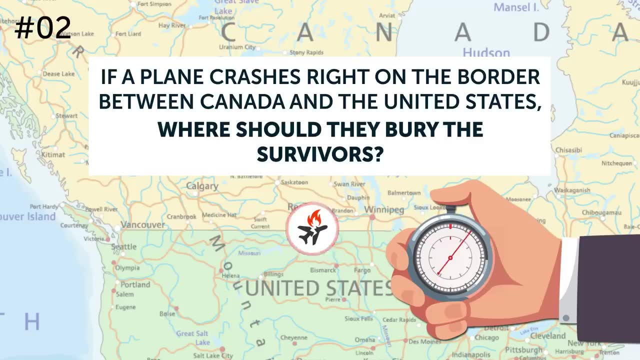 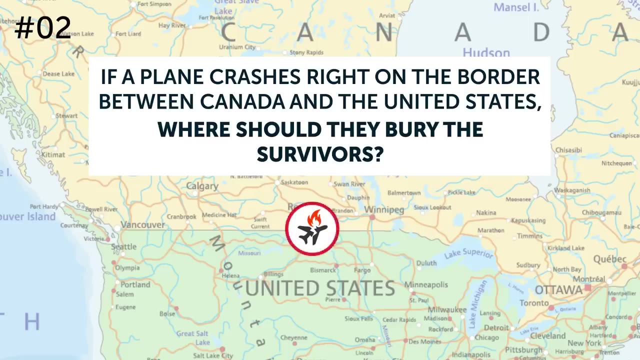 between Canada and the United States. where should they bury the survivors? Whoa? are you supposed to know international aviation laws or something? Well, take 10 seconds to figure it out. Have you made up your mind? Canada, USA, Hmm, But are you 100% sure they bury the survivors? 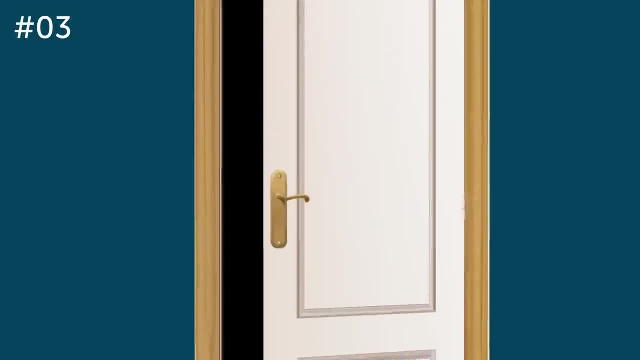 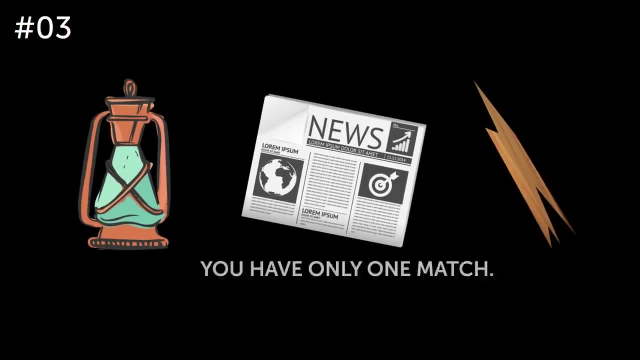 3. Okay, how about this one? Imagine that you just entered a pitch-black room. There's an oil lamp, a newspaper and some kindling wood inside the room, But you only have one match. You have to make a tough choice. You have to make a choice. You have to make a choice. You have to make a. 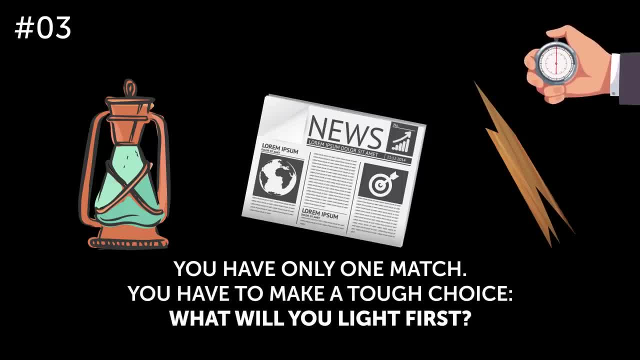 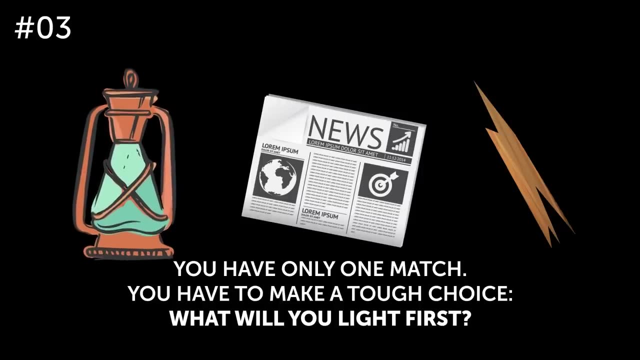 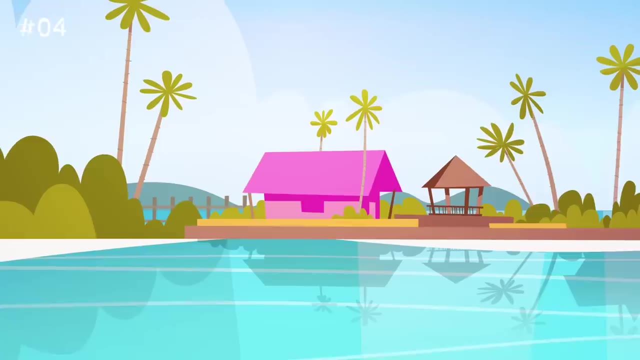 choice. What will you light first? The oil lamp is definitely a good choice, but still incorrect. First of all, you'll need to light the match 4.. Mrs Brownie, despite her name, loves the color pink. Her bungalow is a. 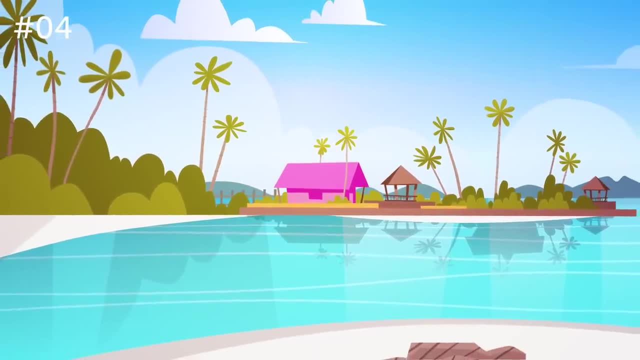 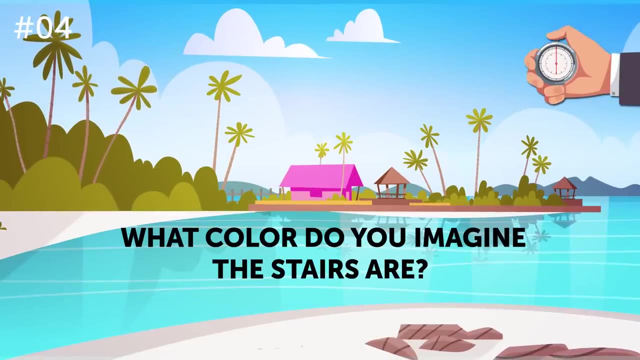 decorated entirely in the bubblegum color: Pink carpet, furniture, curtains, even the walls are pink. So what color do you imagine the stairs are 5.. Perhaps if there were stairs, they would most likely be pink. but bungalows just have one floor, No stairs needed. 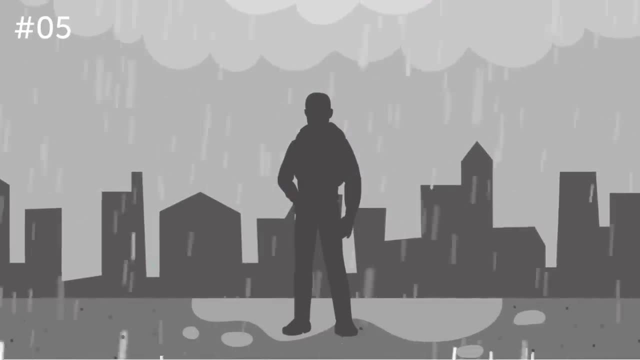 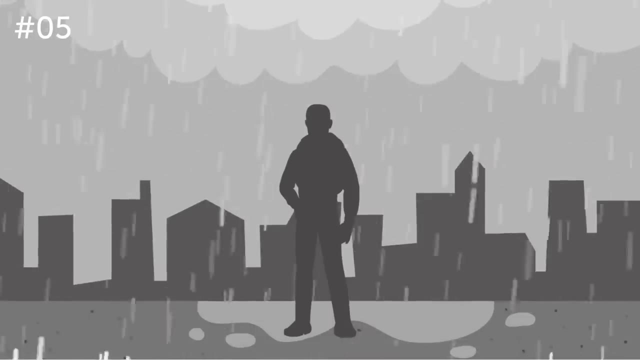 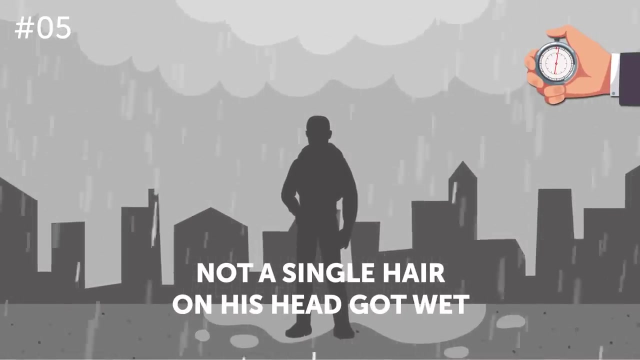 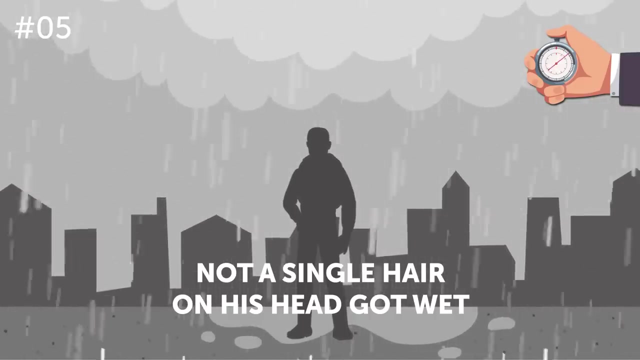 5. One day, a man got caught in the pouring rain. Unfortunately, he had no umbrella or hat or anything else he could use to stay dry, Yet not a single hair on his head got wet. How so? The answer is so simple. you'll want to see it, So let's get started. 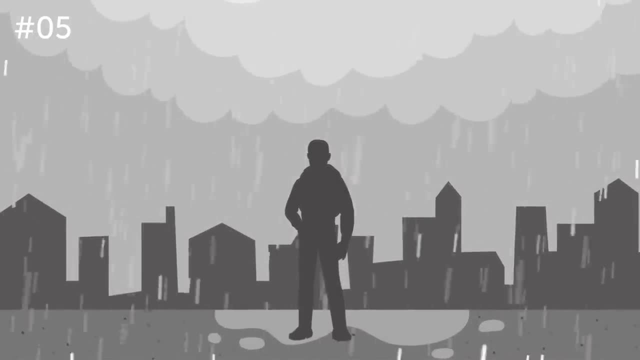 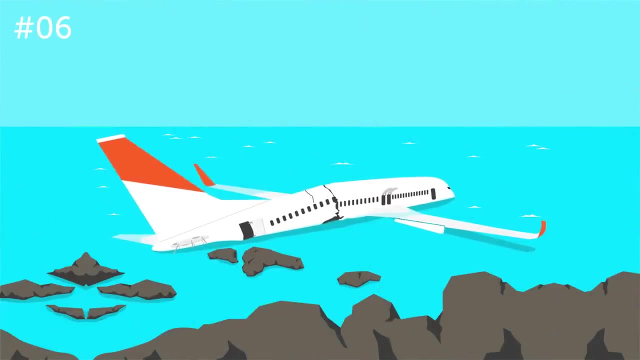 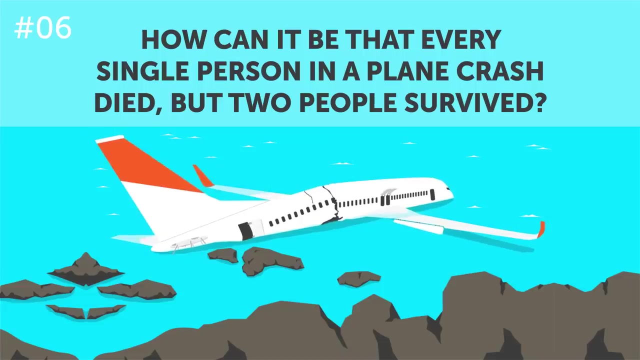 The answer is so simple you'll want to slap yourself for not thinking of it. The man was bald 6.. How can it be that every single person in a plane crash died, but two people survived? This is a straight-up paradox and you have only 10 seconds to explain it. 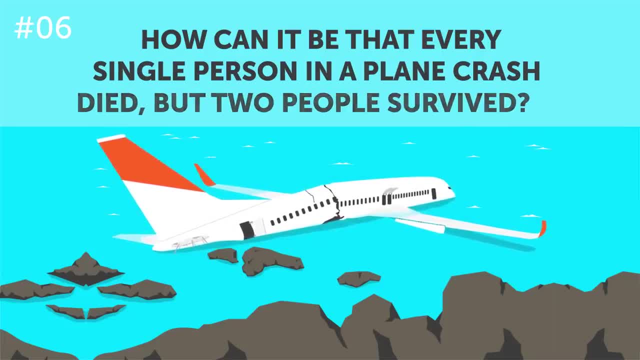 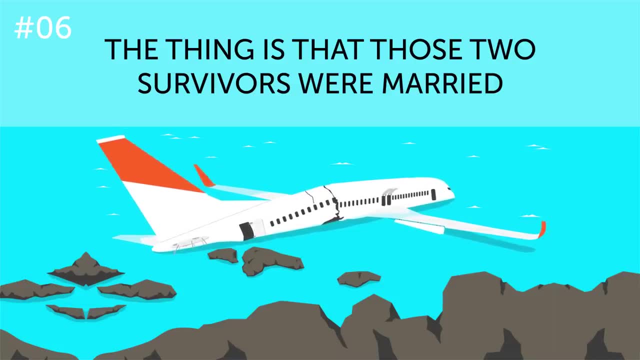 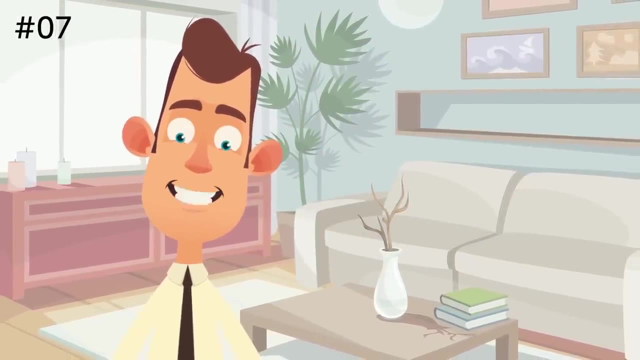 The thing is that those two survivors were married. Every single person. Ah, I see what they did there. 7. Time for a tricky one, so be very attentive. What do you sleep on? sit on and brush your teeth with. 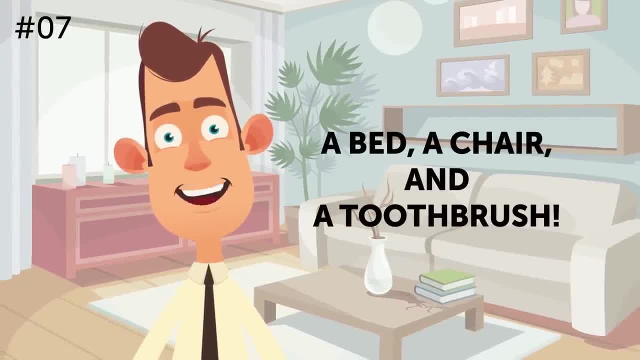 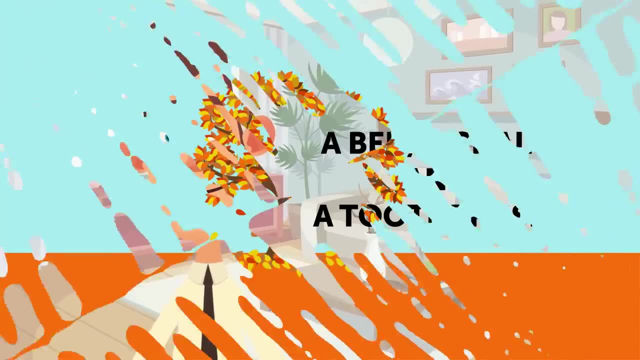 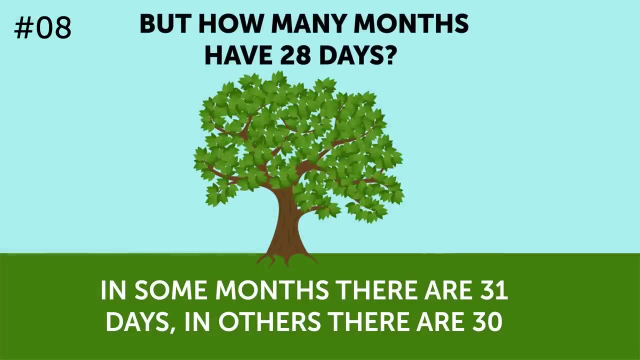 A bed, a chair and a toothbrush. Common sense remember. Don't over-complicate things. 8. In some months there are 31 days, in others there are 30. But how many months have 28 days? 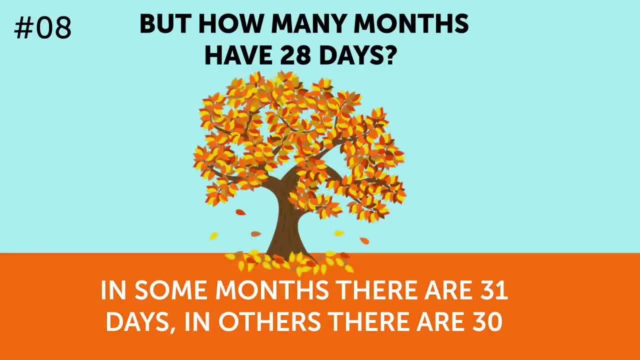 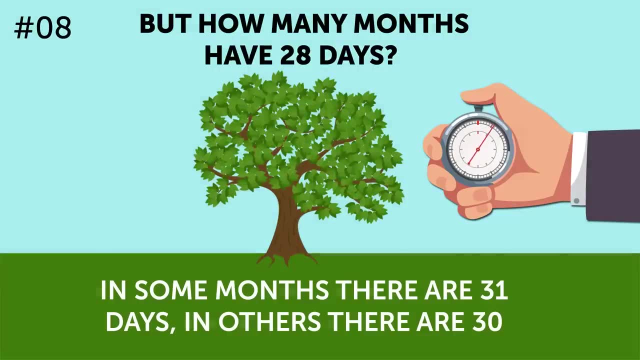 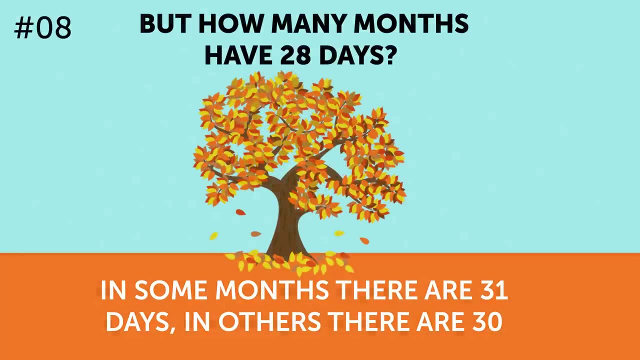 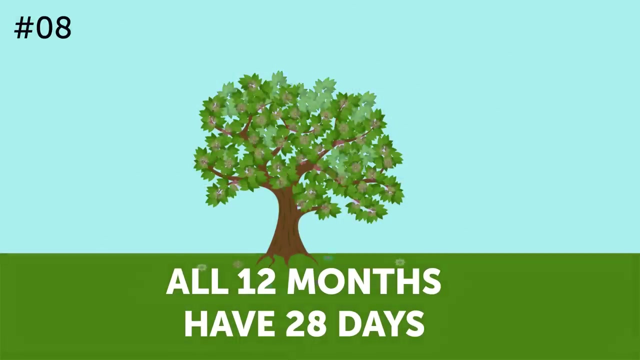 Come on, you know this one. You've got 10 seconds to remember. So is it just one February, right? Nope, The answer is actually 12.. All 12 months have 28 days. Press the like button if you got that one. 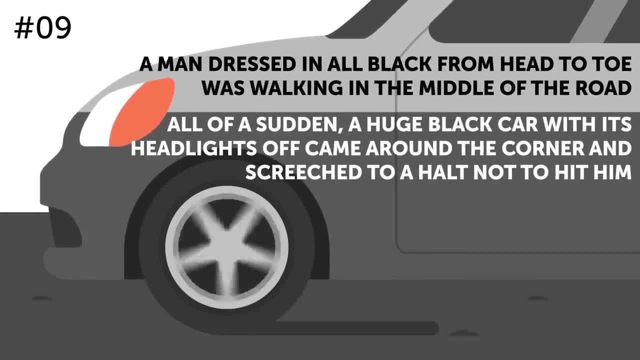 9. A man dressed in all black from head to toe was walking in the middle of the road. All of a sudden, a huge black car with its headlights off came around the corner and screeched to a halt not to hit him. 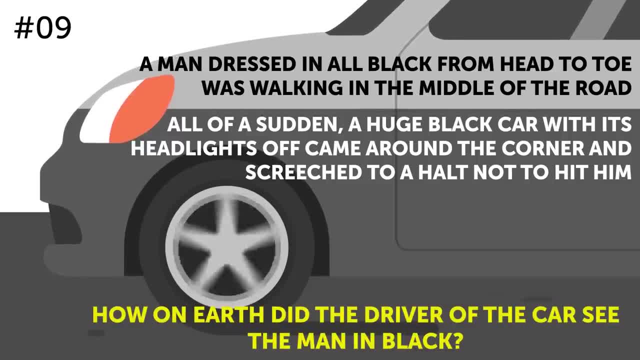 8. How can it be that every single person in a plane crash died, but two people survived? How on earth did the driver of the car see the man in black And 10 seconds on the clock? If you need more time, just pause the video. 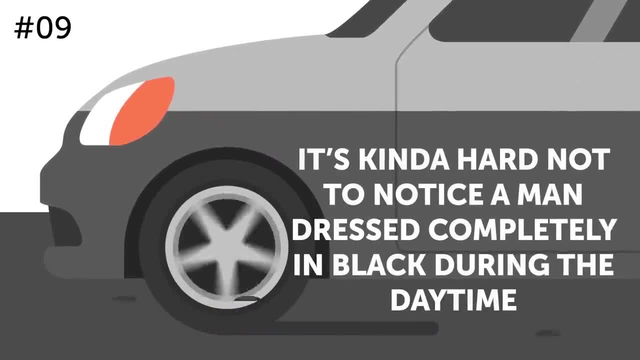 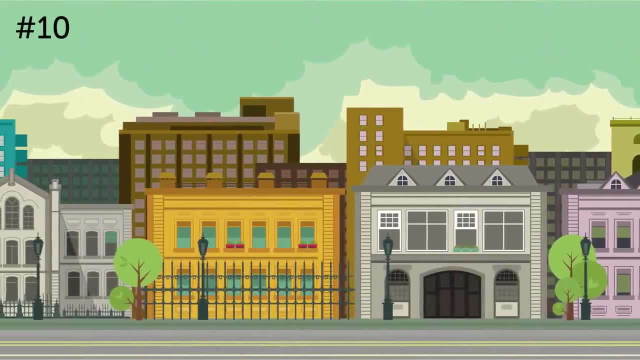 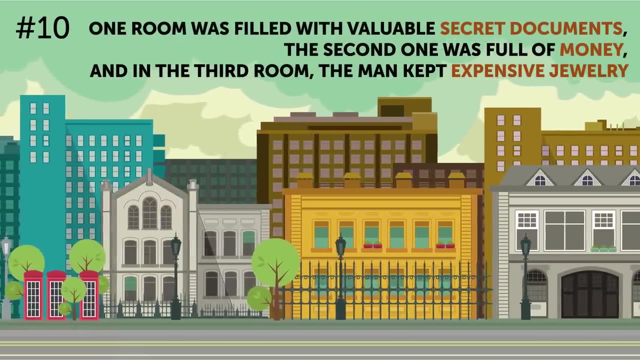 Well, it's kind of hard not to notice a man dressed completely in black during the daytime. 10. There were three houses. There were three highly important rooms in the house of an extremely important man. One room was filled with valuable secret documents, the second one was full of money and in the third room the man kept expensive jewelry. 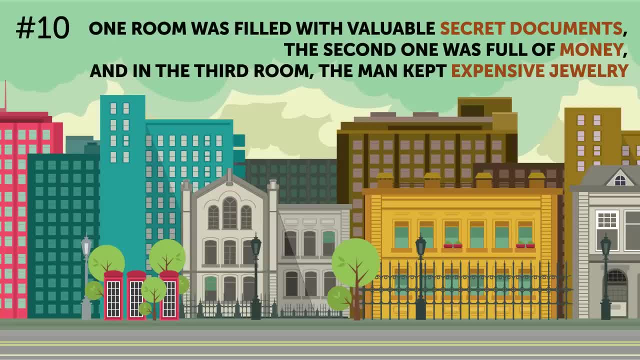 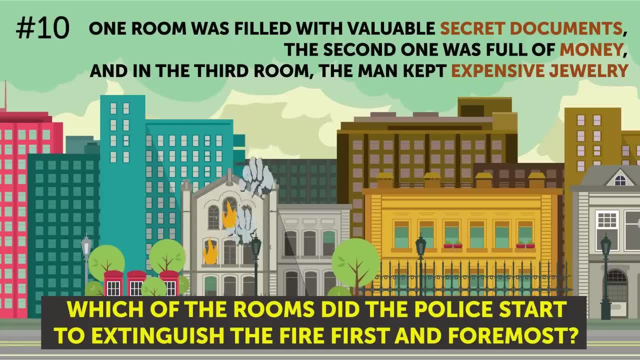 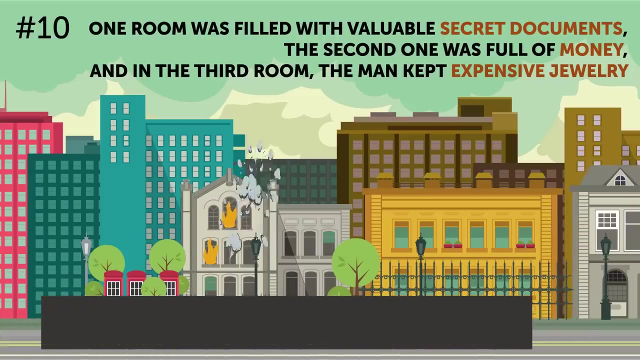 But one day an arsonist set the house on fire and all the highly important rooms burst into flames. Which of the rooms did the police start to extinguish the fire? first and foremost, You can debate the philosophical stuff later, but let's get one thing straight. 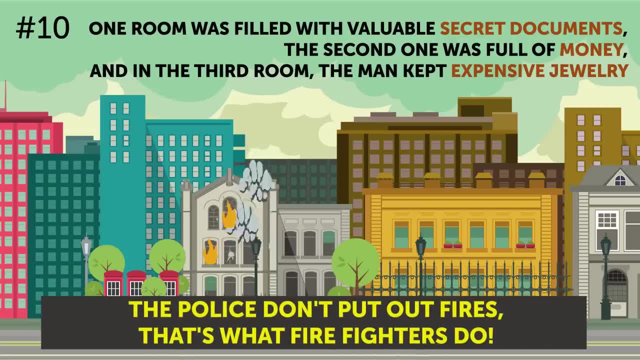 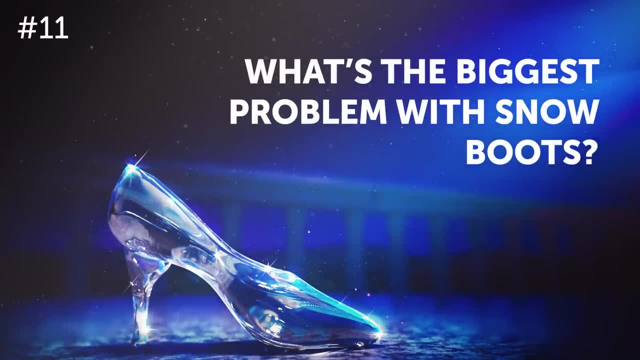 The police don't put out fires. That's what firefighters do. 11. What's the biggest problem with snow boots? That's a pretty random question. Still, take 10 seconds to think of your complaints about this winter weather must-have. 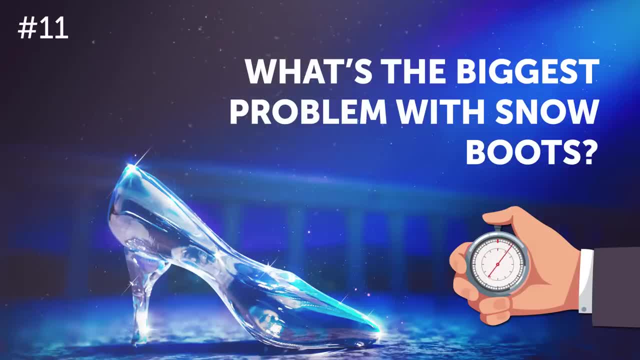 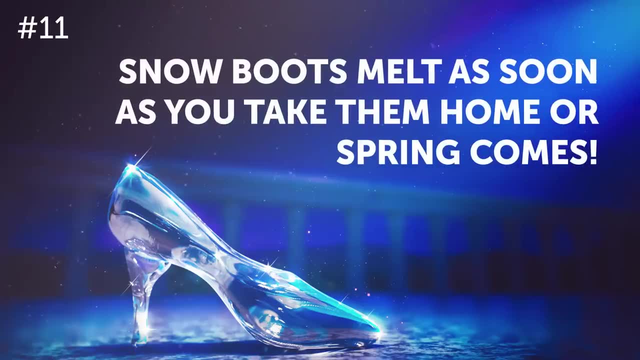 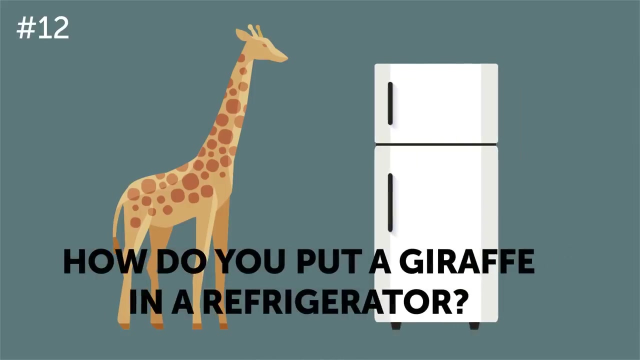 Snow boots melt as soon as you take them home. or spring comes. Oh, because these ones are made of snow. Gotcha 12.. How do you put a giraffe in a refrigerator? You can put a giraffe in a refrigerator, but you can't put a giraffe in a refrigerator, so you have to put a giraffe in a refrigerator. 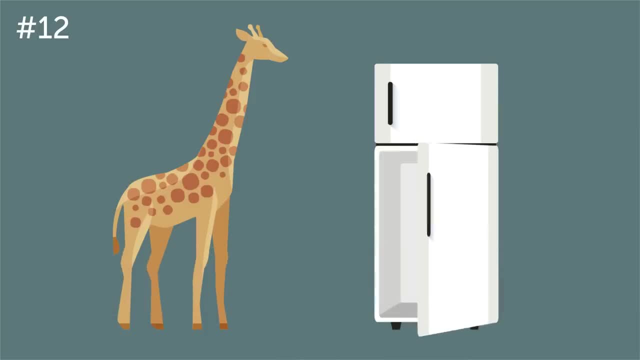 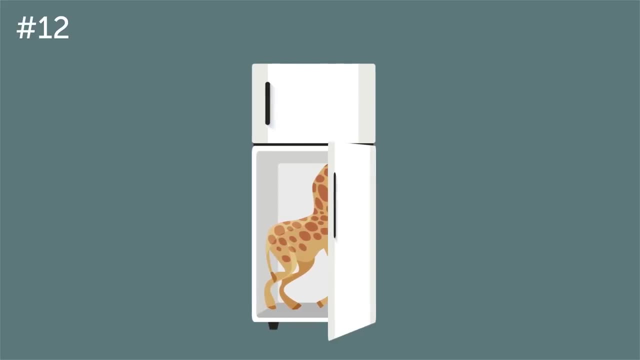 So here's exactly how you do it: You open the fridge and put the giraffe inside. Then it's better to close the door so you won't let the cold out. This question in particular shows if you tend to overcomplicate things. 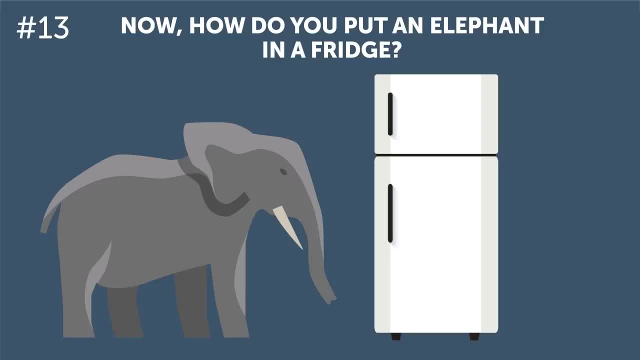 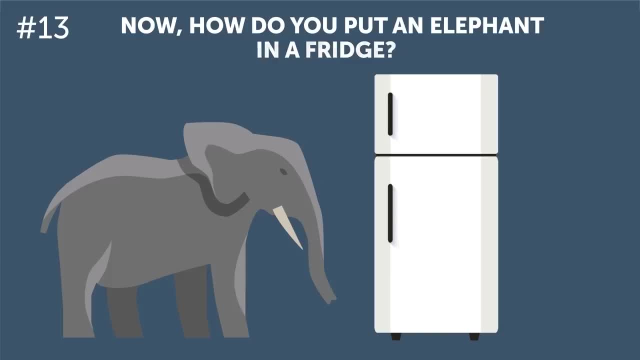 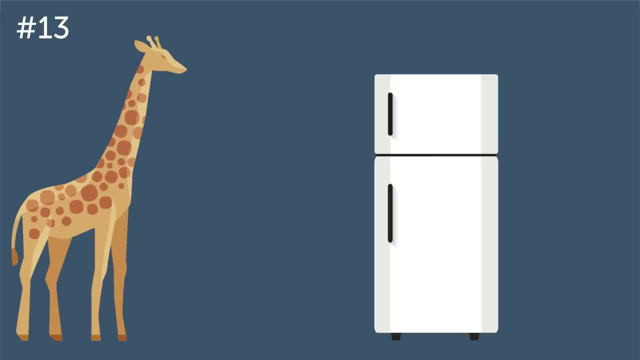 You can't put an elephant in a fridge. Alright, listen carefully. Open the fridge, take the poor frozen giraffe out, put the elephant in and close the door. If you remember the giraffe, you're good at thinking about repercussions of your actions. 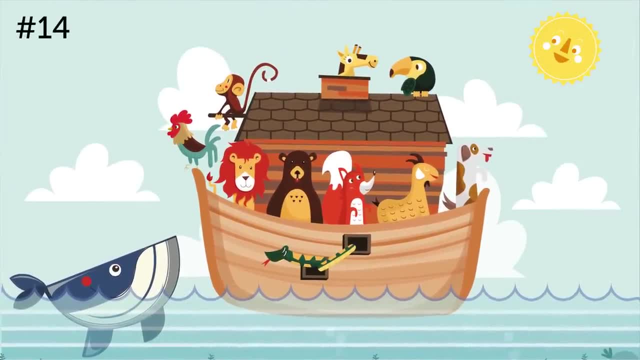 14. Noah builds one more ark and invites all the wolves to come. 14. Noah builds one more ark and invites all the wolves to come. He invites all the world's animals to join him. 14. Noah builds one more ark and invites all the wolves to come. 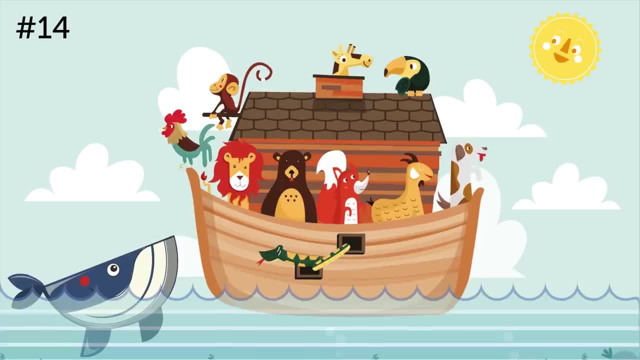 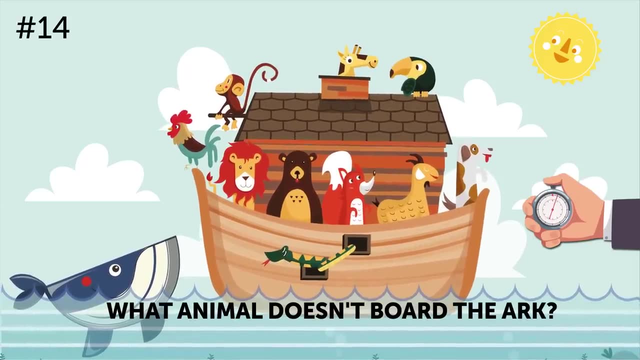 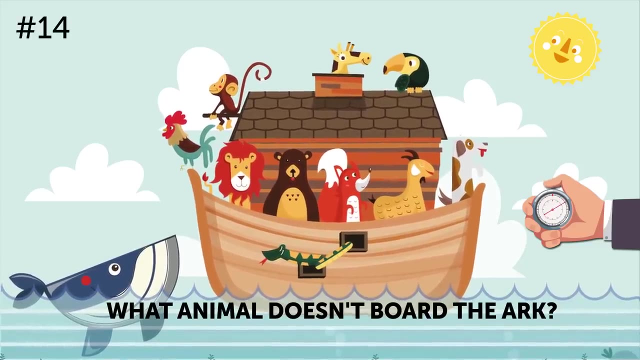 He invites all the world's animals to join him. Every single animal gets on board except for one. Every single animal gets on board except for one. What animal doesn't board the ark? What animal doesn't board the ark? It's the elephant, of course. 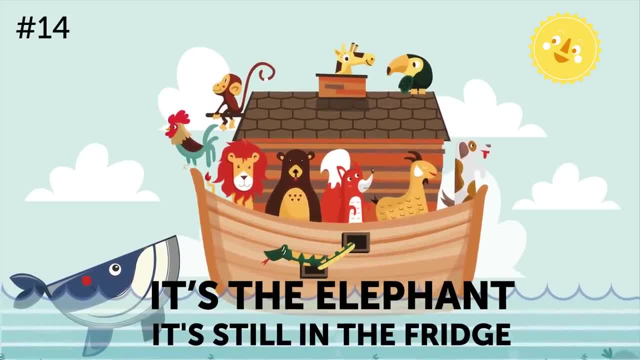 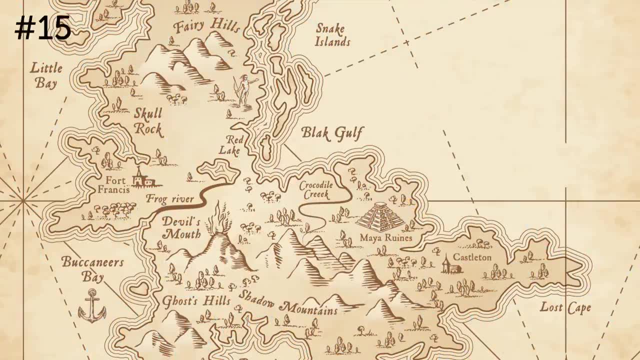 It's still in the fridge. poor thing If you got this one right. your memory is razor sharp. Very nice. 15. You're hiking in the wilderness. when you come upon a river, You have to cross it, but you know that crocodiles dwell in rivers there.